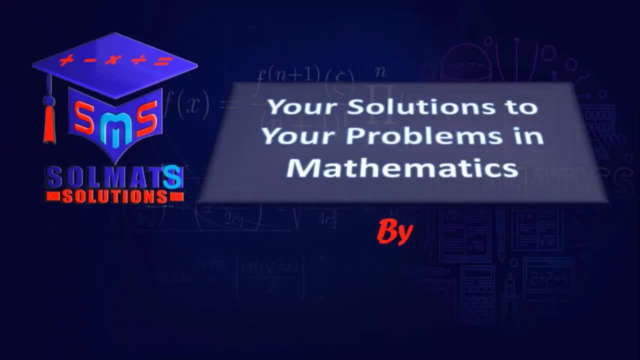 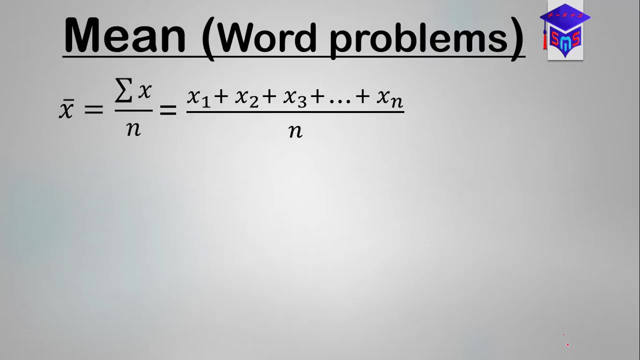 We've been talking about the mean of a set of numbers or the average of a set of numbers. Now we are going to make some important deductions that will help us to be able to solve some more complicated questions. And so if you have a set of data like this and you want 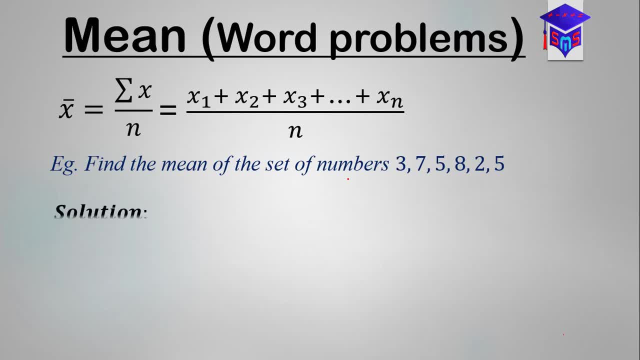 to find the mean. just like the formula goes, we say that the mean is going to be the sum of all the data values divided by the number of data values, which is 6.. And then that is going to simplify to give us 5.. So when you look at this, we are saying that the mean 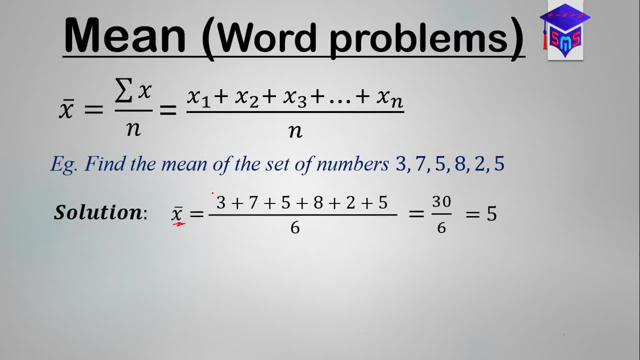 x bar is equal to the sum of all these values divided by the number of data values. divided by this, 6 over. here is the number of values we have. So in simple terms we can say: the mean x bar is equal to the sum of the x values, okay, or the sum of the data values divided. 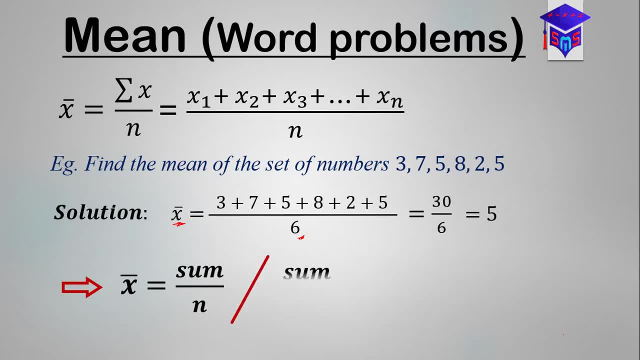 by what? N Or someone can say that the sum of the values over the number of values is equal to the mean or the average. Now this deduction is very important, and then it's going to help us to be able to answer some more interesting questions. 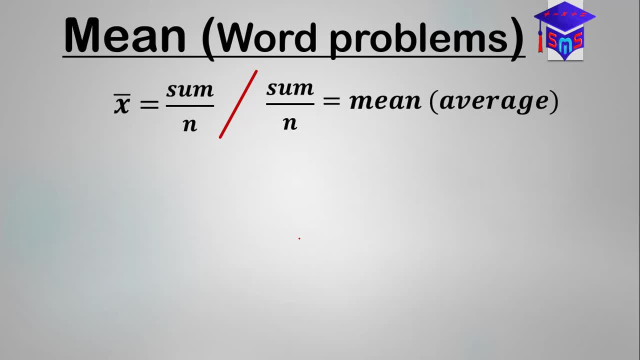 So let's go ahead and then pick some examples like that. Now, if you have a question which is telling you that the average age of 5 men is 47, find the sum of their ages Alright. so with the important deduction we just made, we can go ahead and say that the sum over 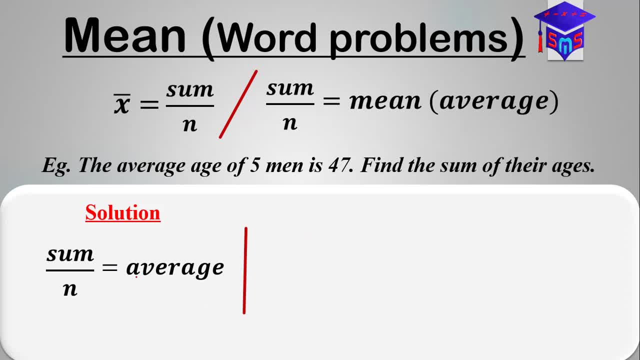 the number of values is equal to the average. Now, this is the average you have over here. So the sum of their ages has been given in the question to be what 47. And then the N we have over here has also been given to be what 5.. So you can substitute and have. 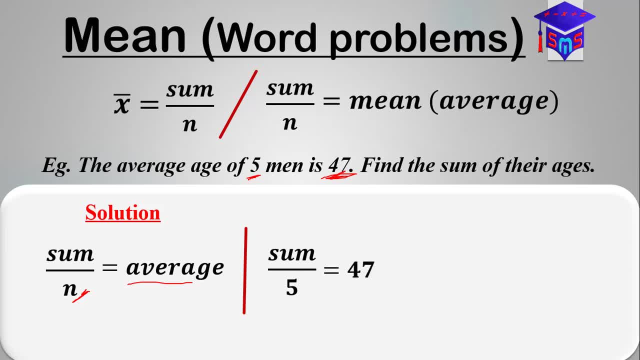 the sum over 5 is equal to the average, which is what 47. So you can solve this. Then you will be having the sum is equal to 47 times 5 and that will be giving us what 235.. Okay.